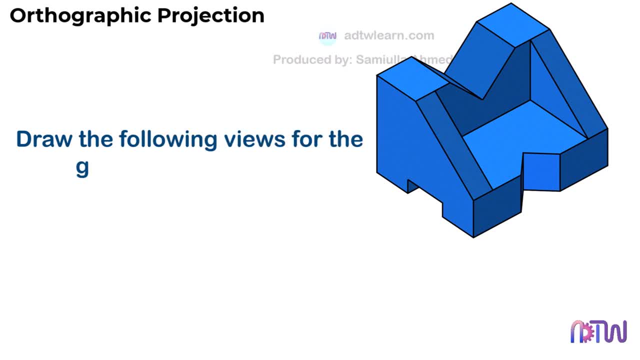 Instructions are as follows: Draw the following views for the given isometric view: Front view looking from x direction, Top view And side view. This given view of the object is called the isometric view. Here we can see the object drawn in a three-dimensional view. 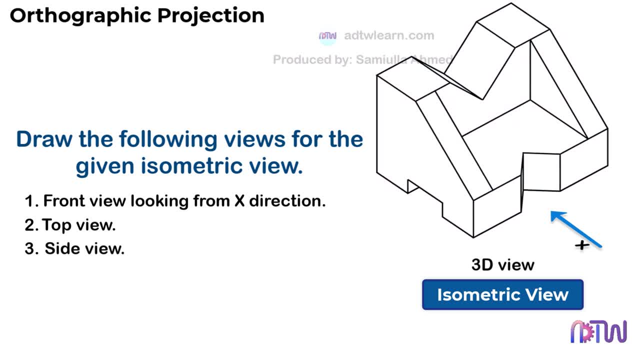 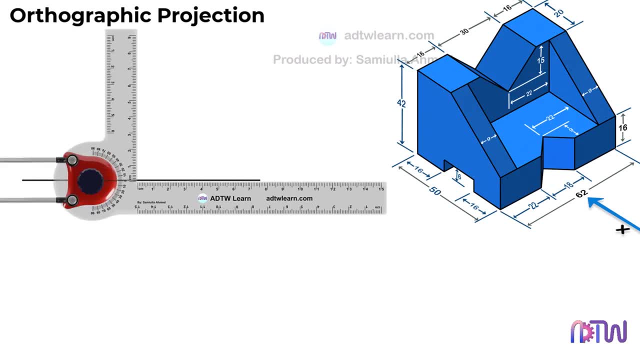 By looking at this view, we have to draw a two-dimensional view of the object. Before drawing, we need to draw the reference lines. Since there are no instructions are given for whether to draw using the first angle or third angle method, we will draw the orthographic view using the first angle method. 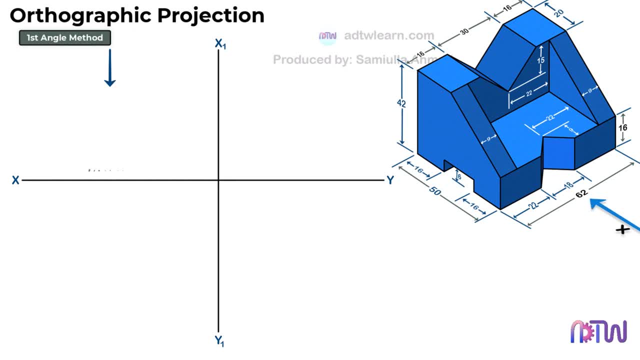 In the first angle method, the front view of the object will be above the xy line and the top view will be below the xy line. The left-hand side view of the object will be on the right-hand side. That is here The viewing direction is given, from this side. Therefore. 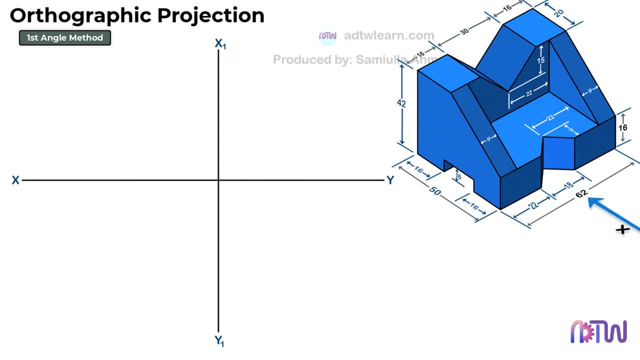 whatever portion of the object is visible while looking from this side will be the front view of the object and it will be drawn above the xy line. And whatever view is visible while looking from this side will be the left side view of the object which will be drawn here. Suppose: 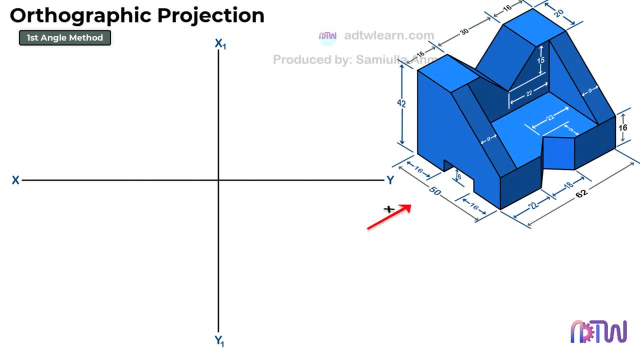 the viewing direction was given on this side, then this view would have been the front view of the object and this view would have been the right-hand side view of the object. In that case, the front view, which is this view we would have drawn here, and the right-hand 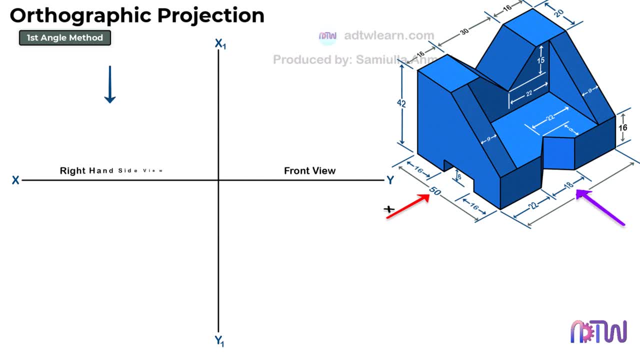 side view, which is the view visible from this side, would have been drawn here, And the top view of the object will always be below the front view. Let's start drawing When we view the object from the direction X. this is how it looks. 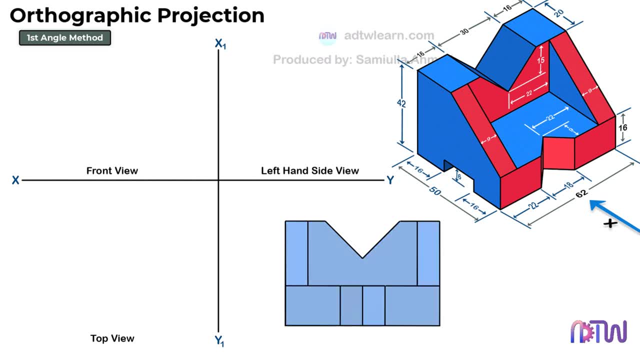 I will color the visible sides on the isometric view for your convenience. We can see the height of the object as 42mm and the total width of the object as 62mm. That is, this 16mm plus this 30mm plus 16mm, which will be equal to 62mm. 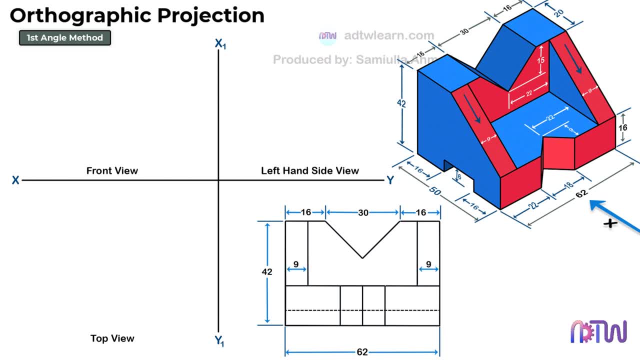 Next, we can see the thickness of these sidewalls as 9mm. The depth of this notch is 15mm and it is 22mm away from this wall. Similarly, the notch provided on this front wall has an 18mm width and its center is: 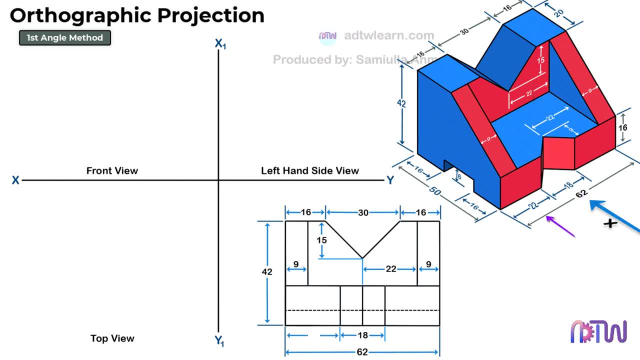 22mm away from this sidewall, And this distance is 22mm. Apart from this, we can see this dotted line. the hidden features of the object are represented by dotted lines. In this isometric view, we can see there is a slot. 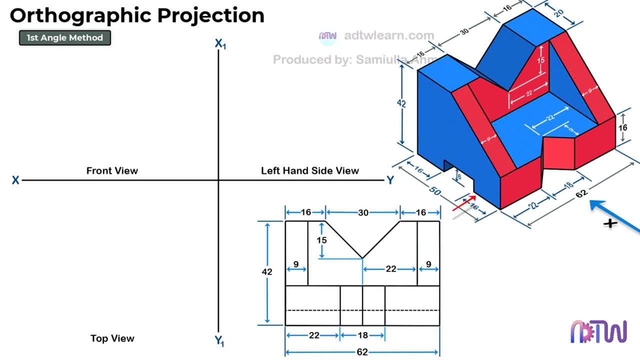 This slot is not visible in the front view because of this front part. in that case, it is represented with the dotted line. The depth of this slot is 6mm. Since we are looking at this figure from the front view, only the depth of this sloth is. 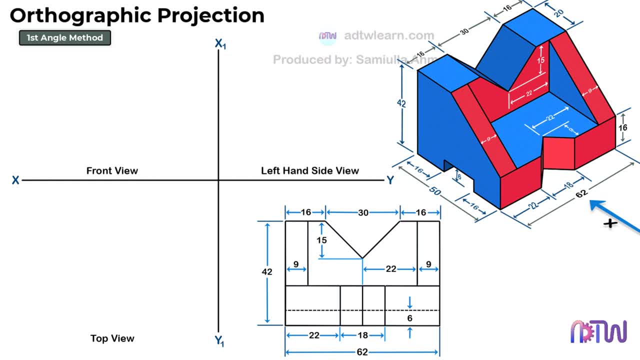 shown by the dotted line. This is the required front view of the object. Let's start drawing. Take a drafter and draw a horizontal line of 62mm And draw a vertical line of 42mm from the end points of this line. 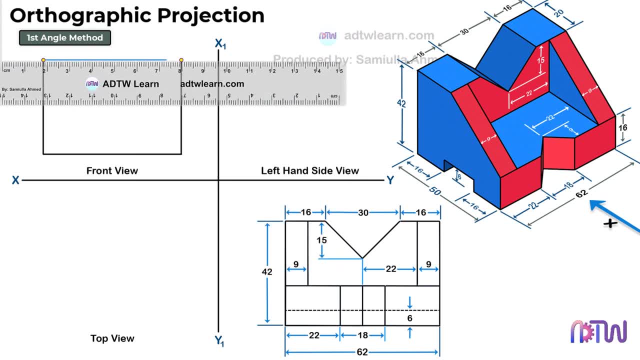 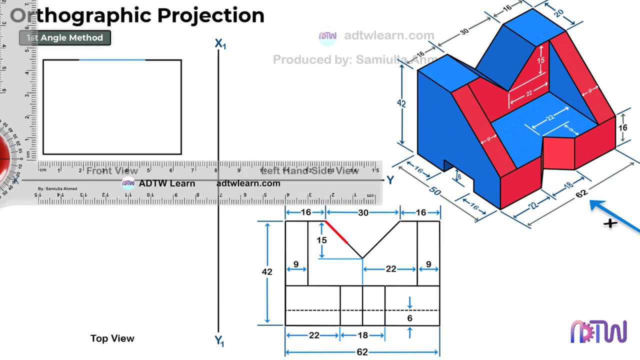 And join these two points with a light line We can see. the length of these lines is 16mm. Therefore, take a drafter and draw a horizontal line of 16mm from these two points. as shown We can see, this notch is in the center of this object. 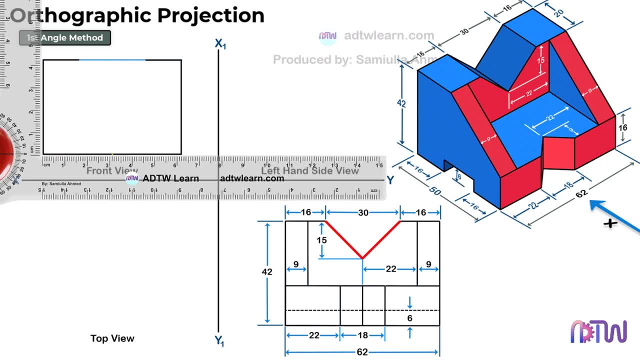 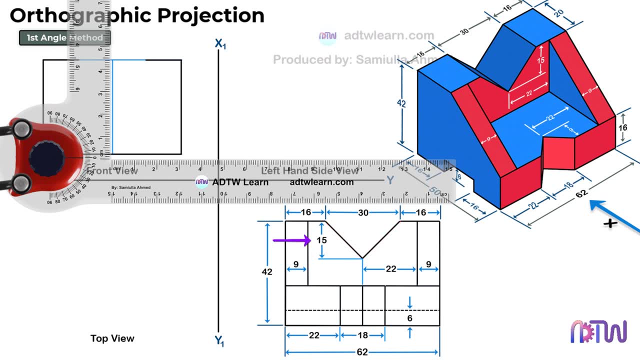 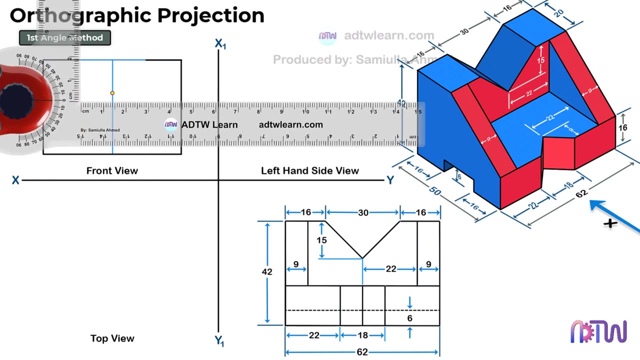 Therefore, mark a point on this horizontal line And draw a light vertical line from this point. We can see the depth of this notch is 15mm And draw a horizontal line of 16mm from this point. Therefore, mark a point at 15mm from the top on this vertical line. 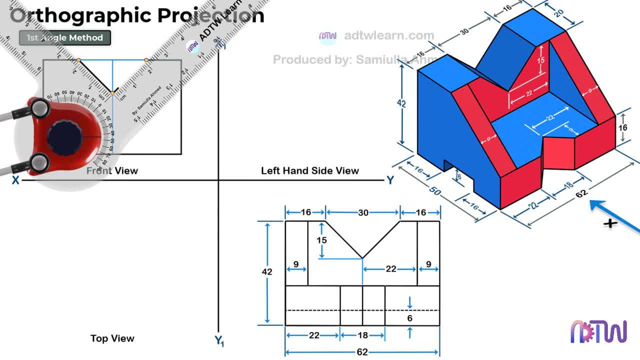 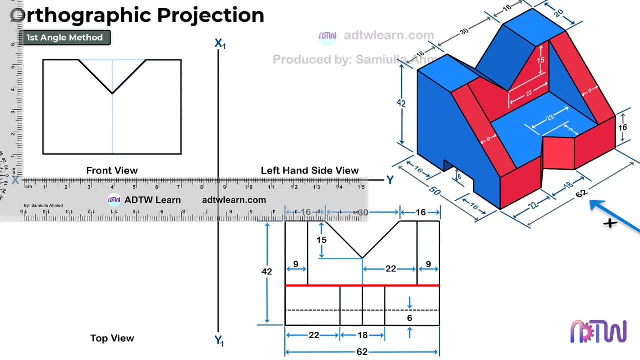 After this, join these points. We got the outline of the object. Next, we will draw this horizontal line. The distance of this line from the bottom is 16mm. Mark 16mm from the bottom on this vertical line And draw a horizontal line from this point. 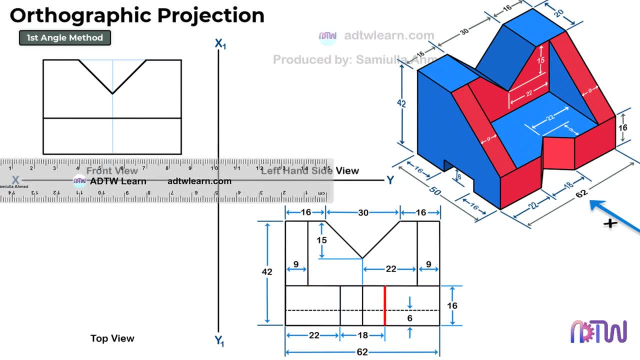 We can see the distance between these lines is 18mm, Which means each of these lines is 9mm away from the center. We can see the distance between these lines is 18mm, Which means each of these lines is 9mm away from the center. 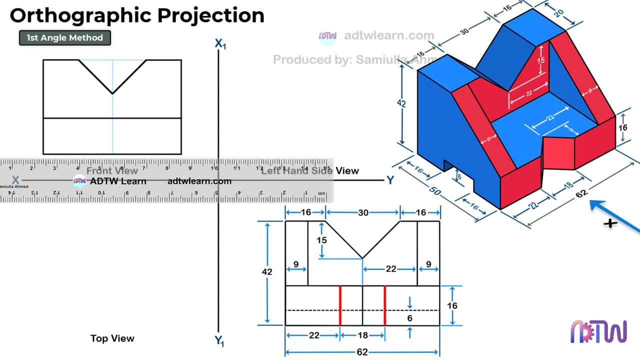 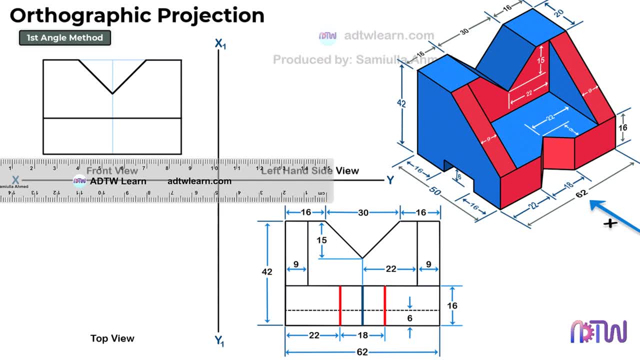 Which means each of these lines is 9mm away from the center. We can see the distance between these lines is 18mm, Which means each of these lines is 9mm away from the center. We can see the distance between these lines is 18mm. 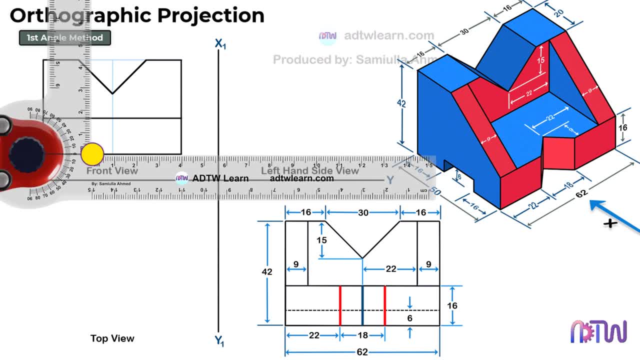 Which means each of these lines is 9mm away from the center. We can see the distance between these lines is 18mm, Which means each of these lines is 9mm away from the center, Which means each of these lines is 9mm away from the center. 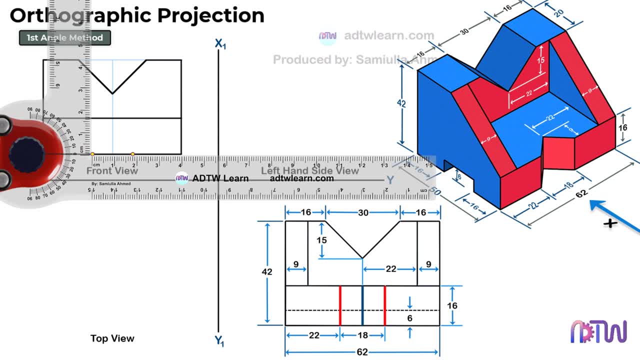 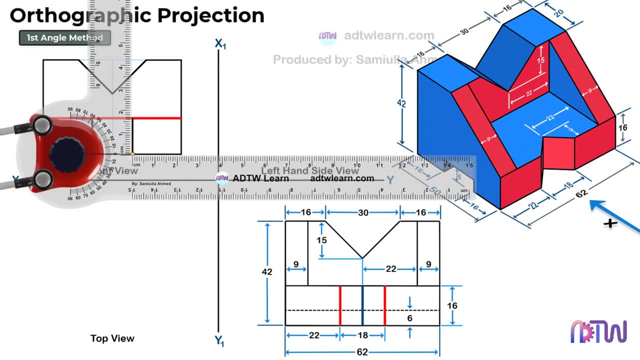 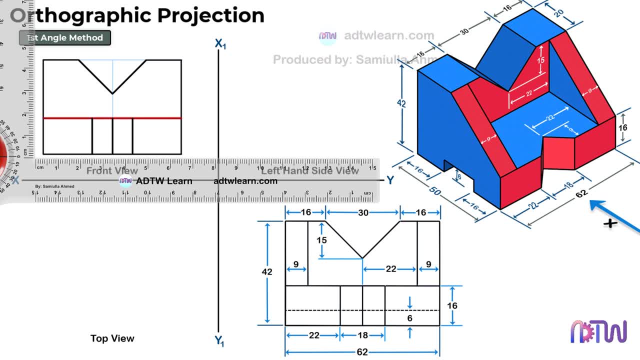 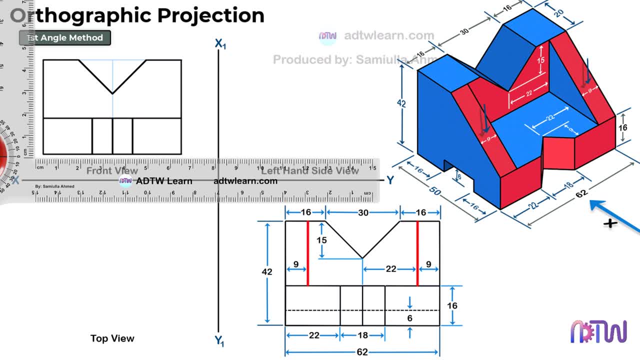 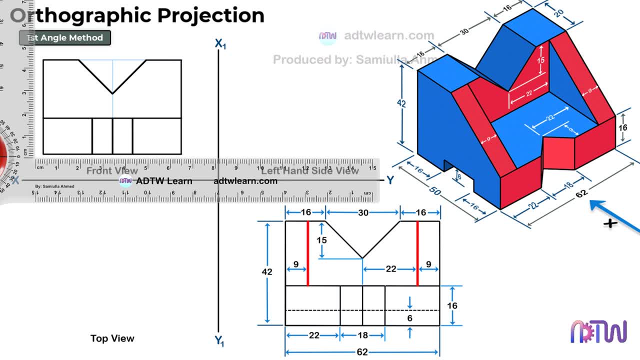 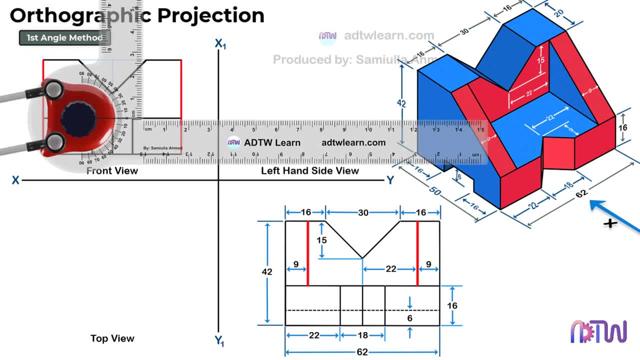 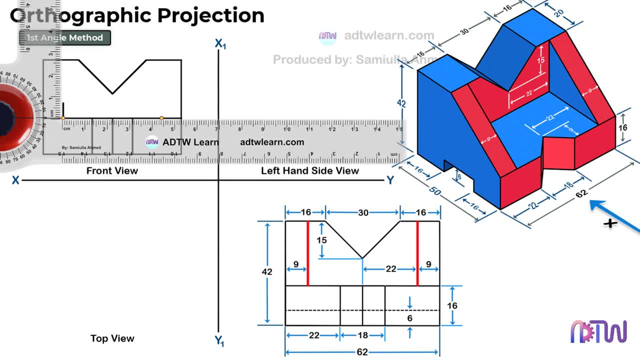 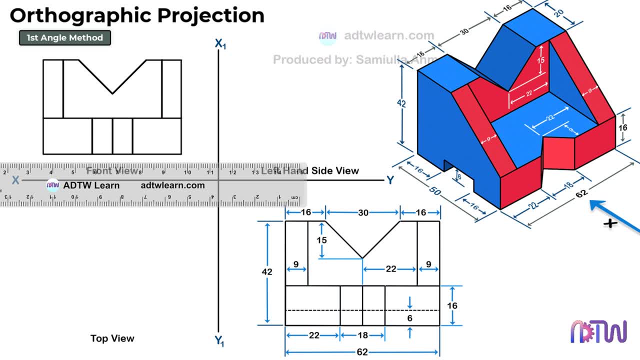 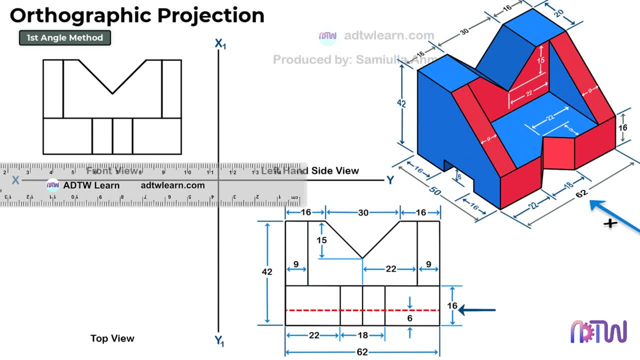 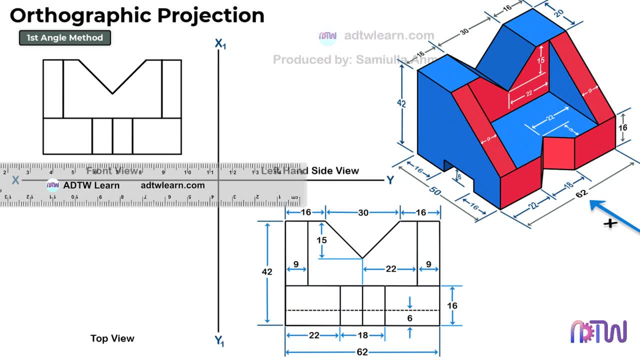 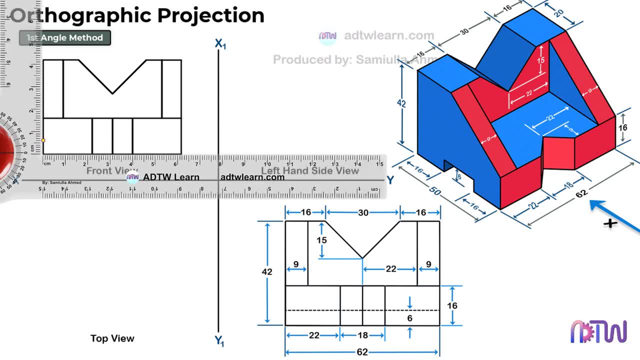 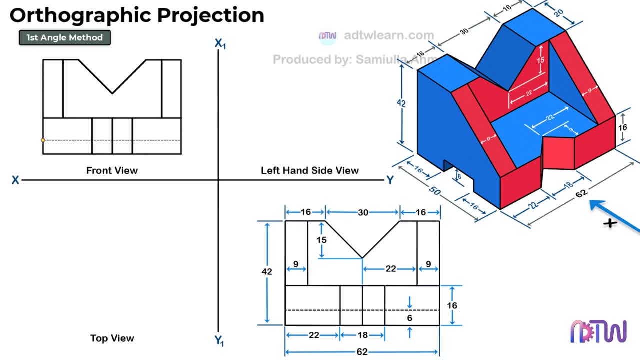 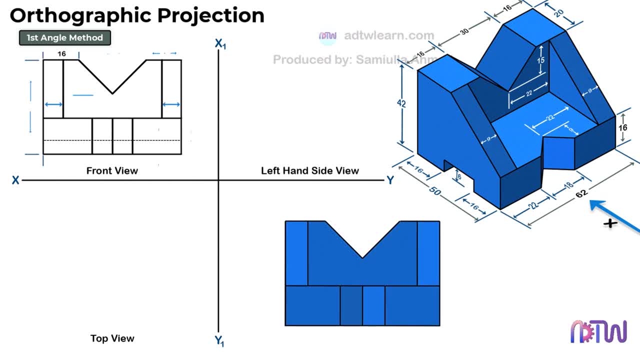 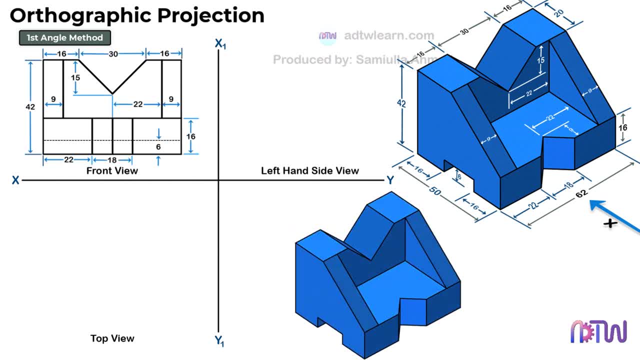 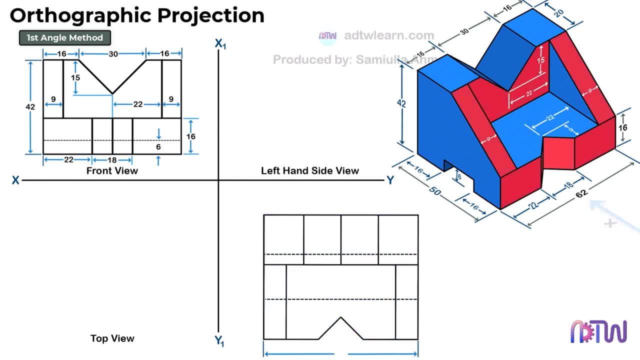 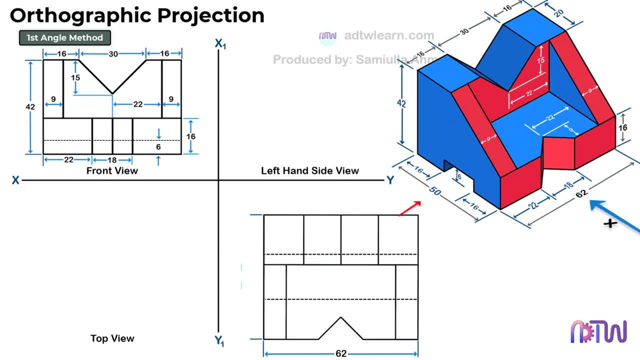 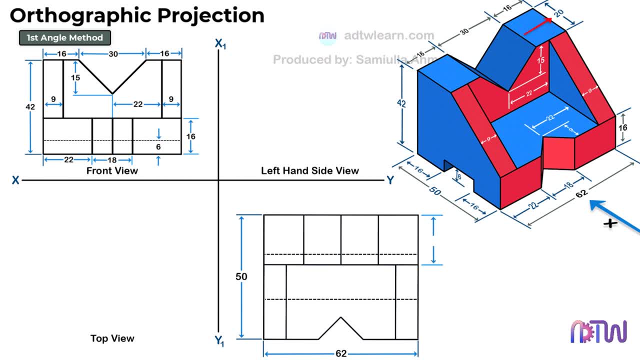 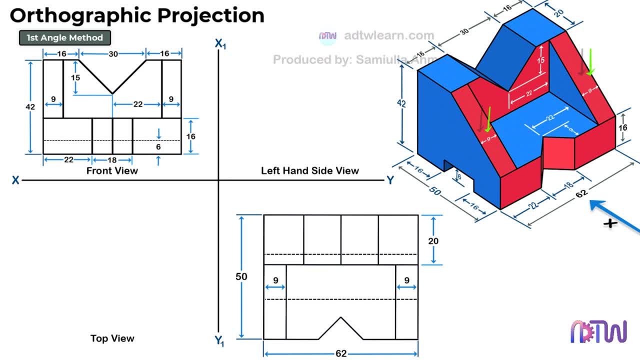 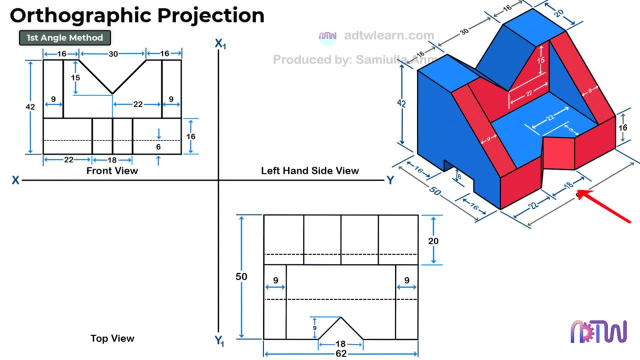 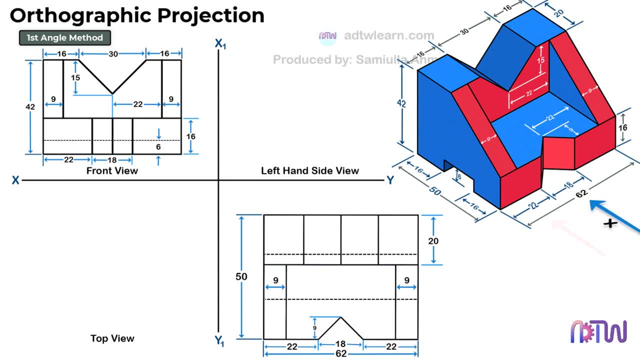 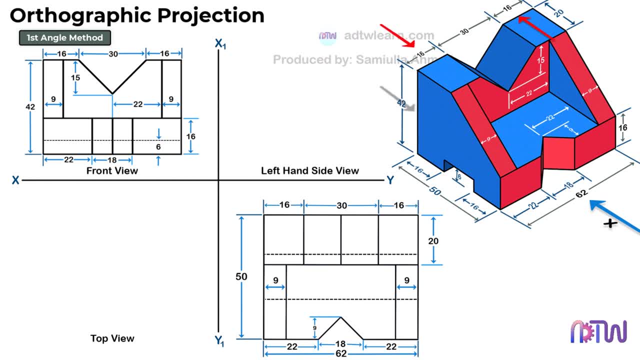 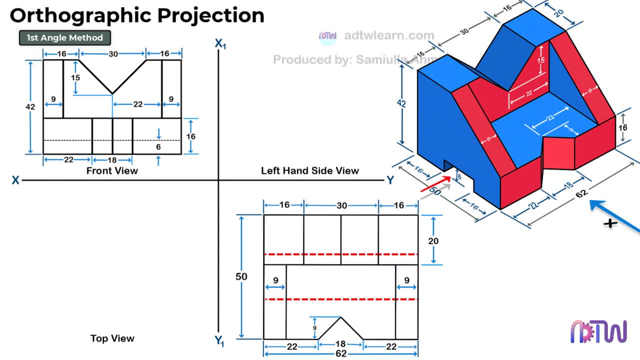 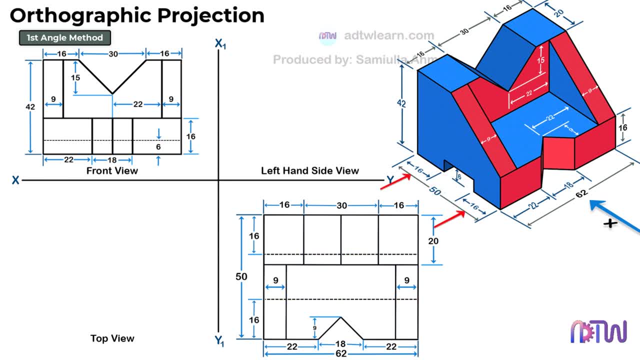 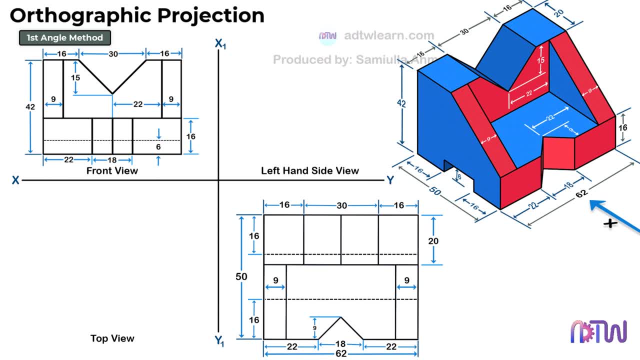 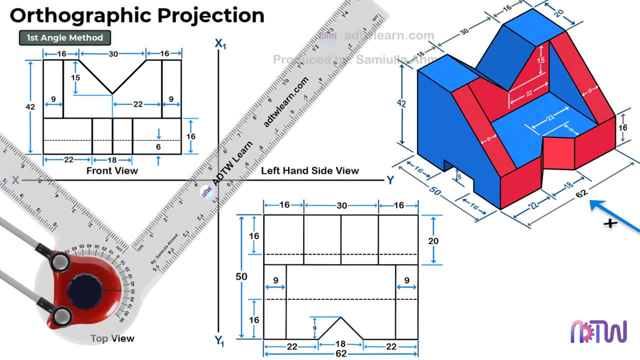 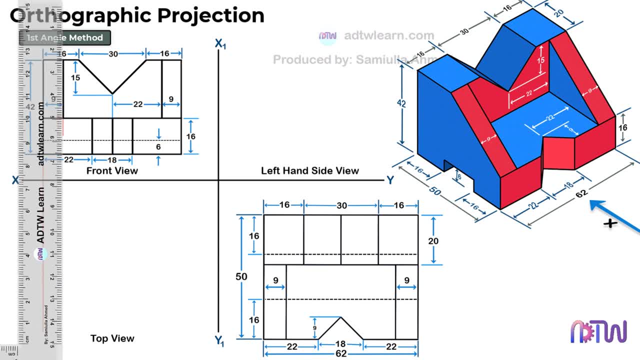 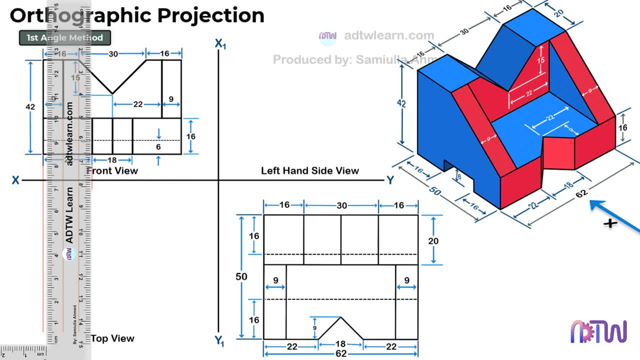 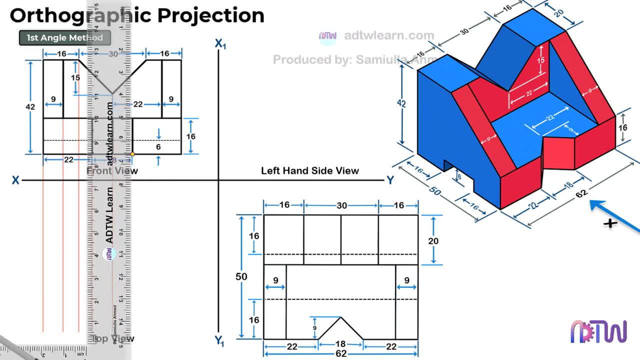 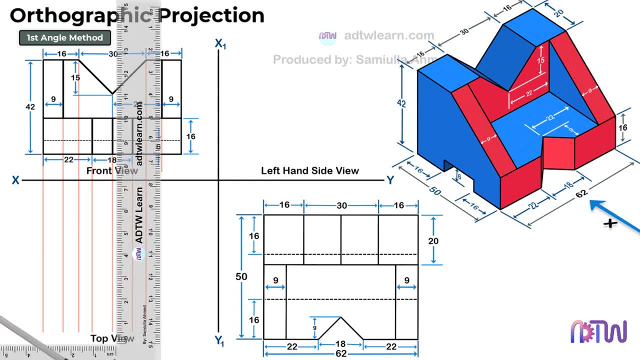 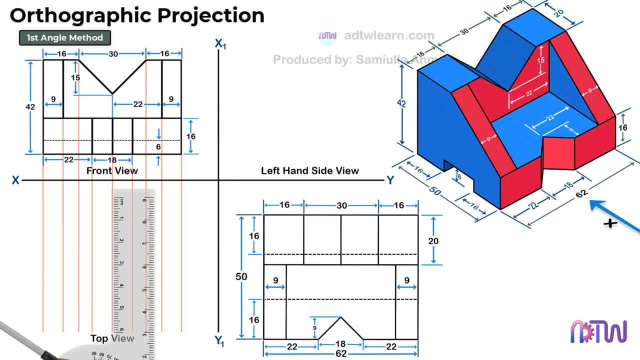 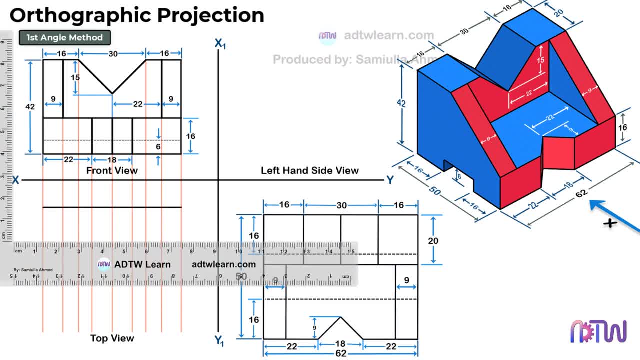 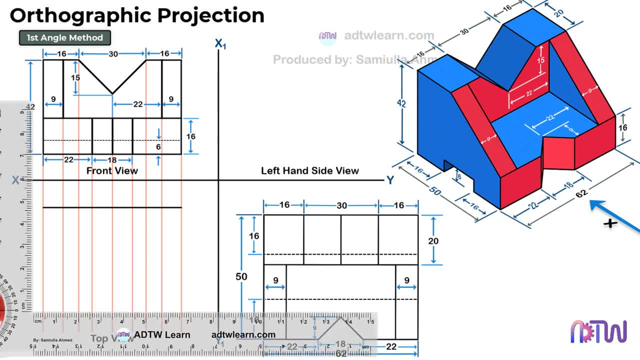 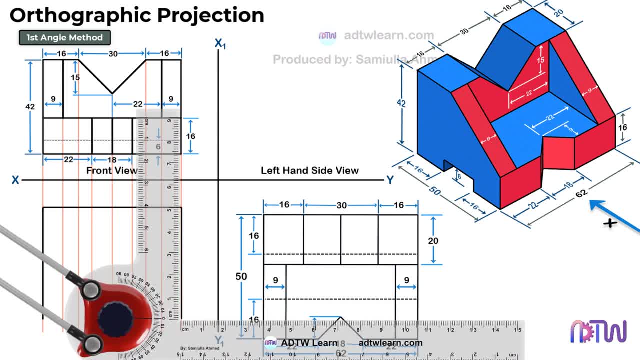 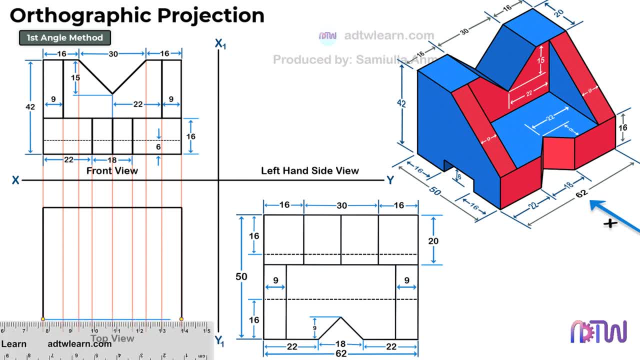 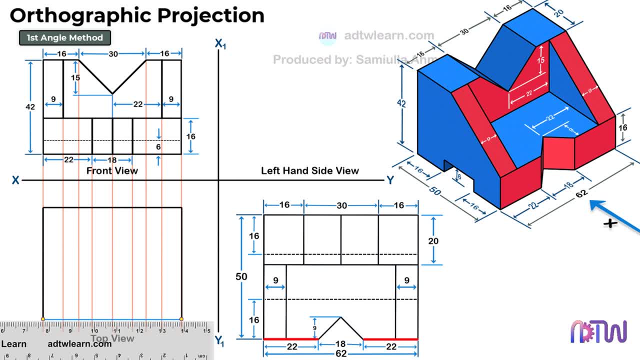 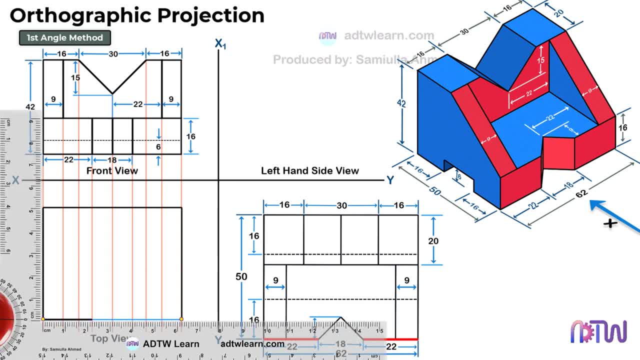 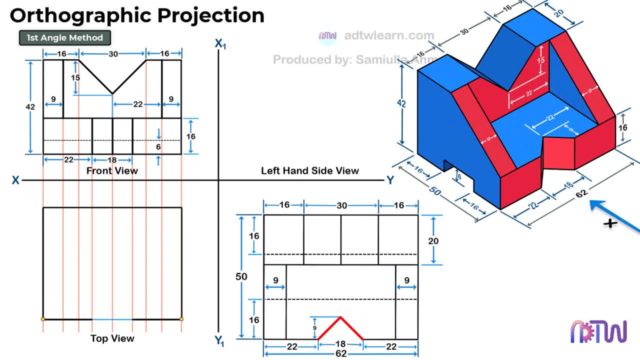 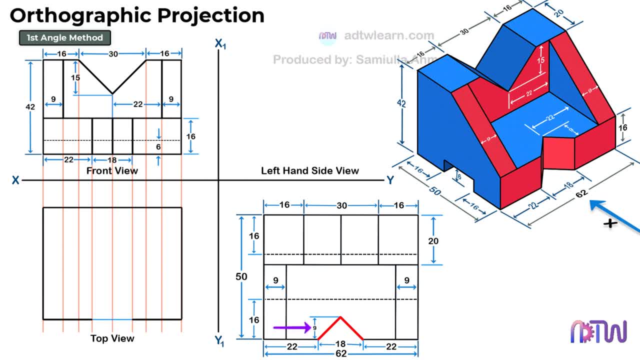 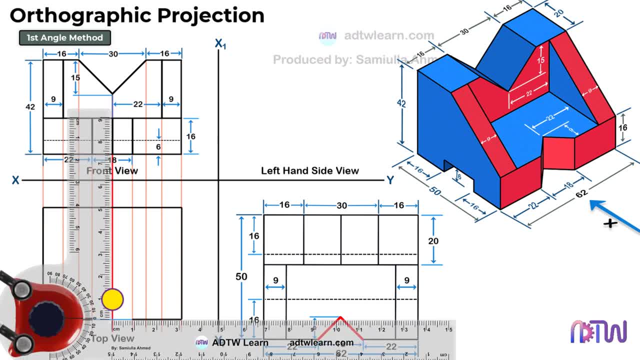 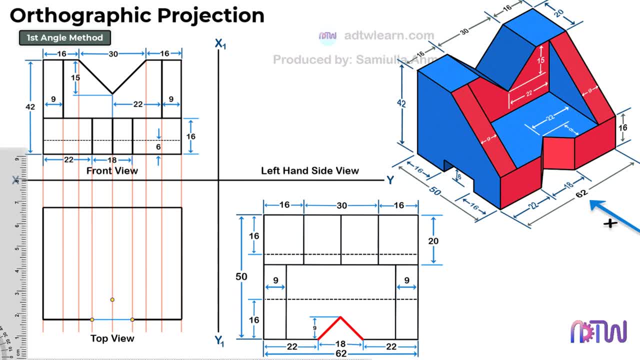 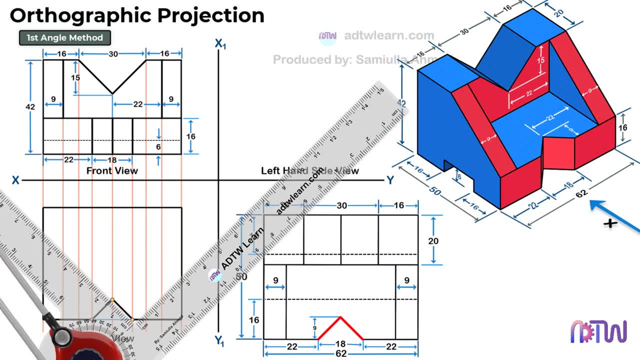 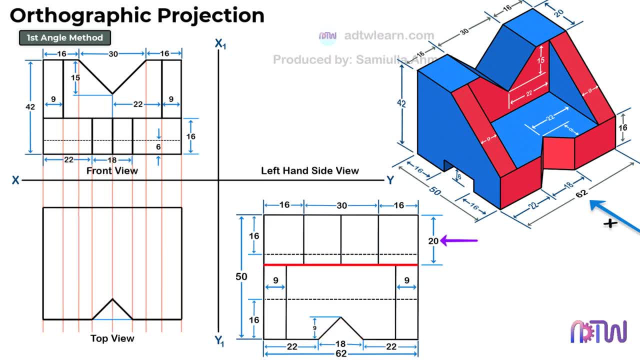 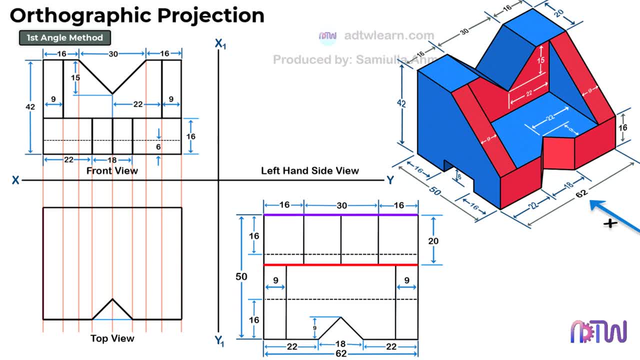 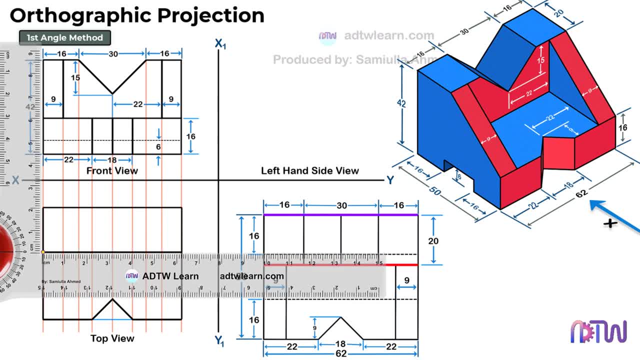 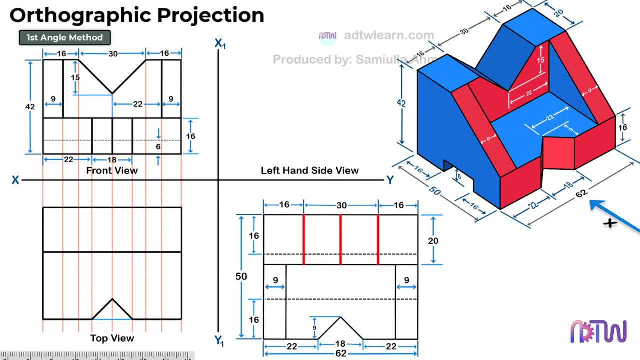 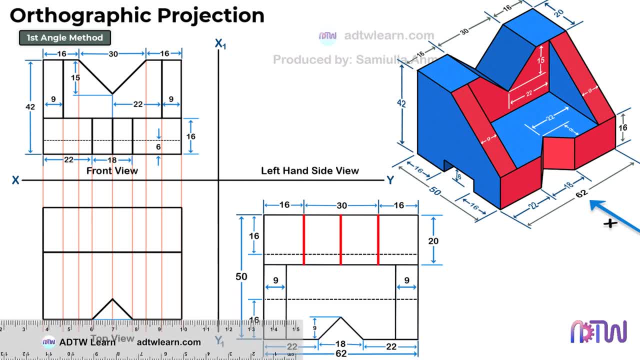 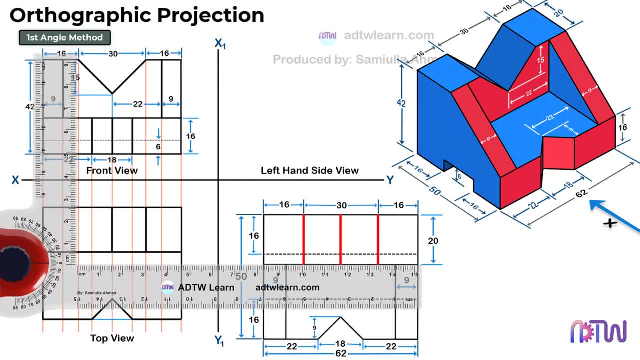 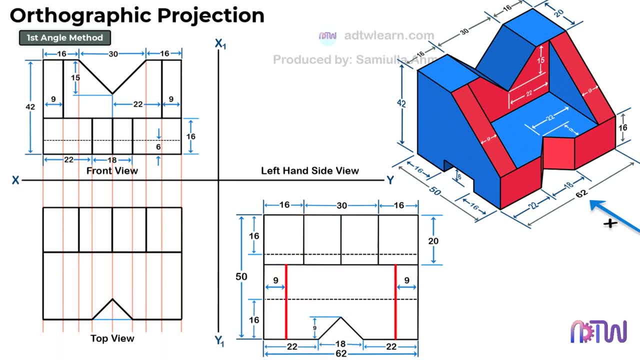 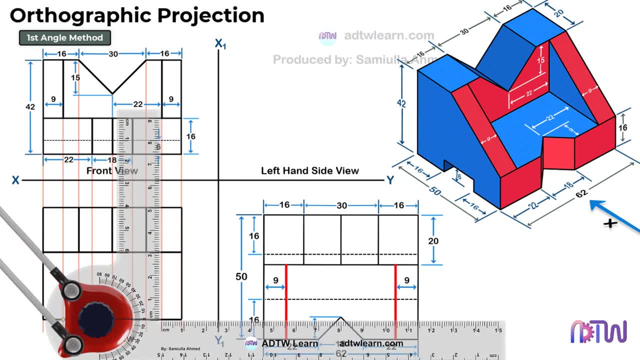 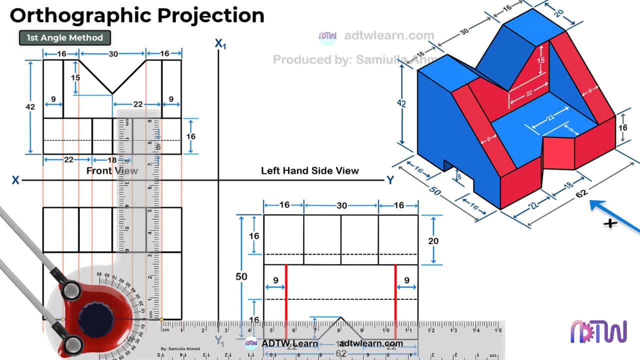 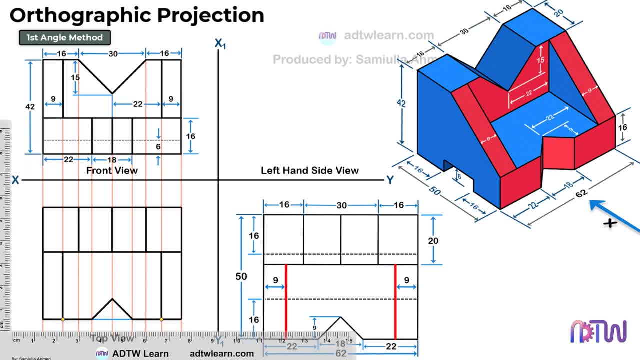 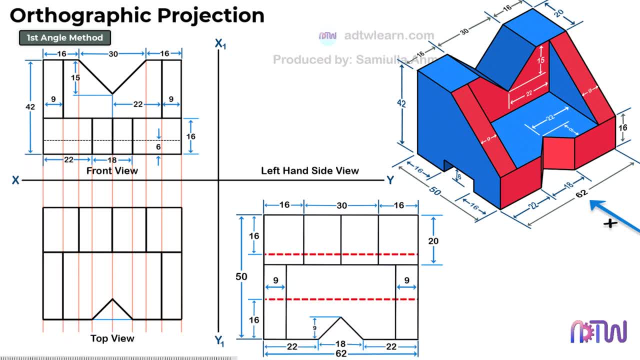 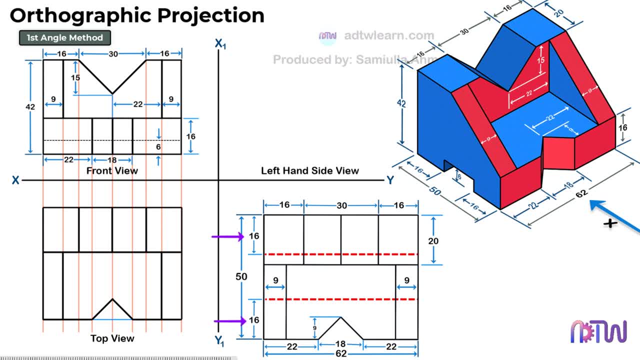 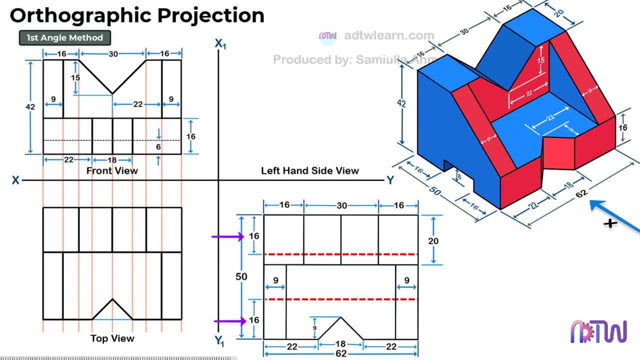 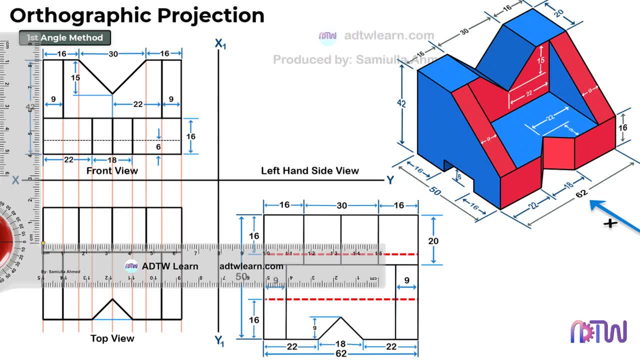 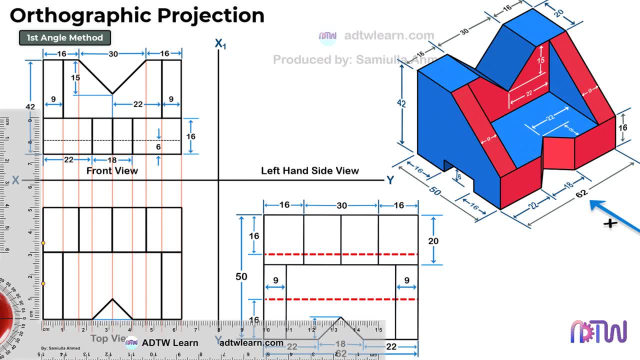 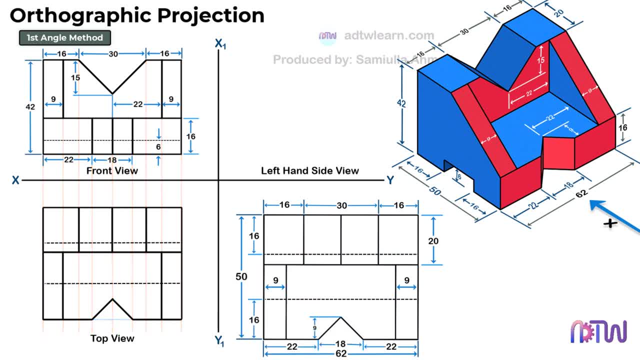 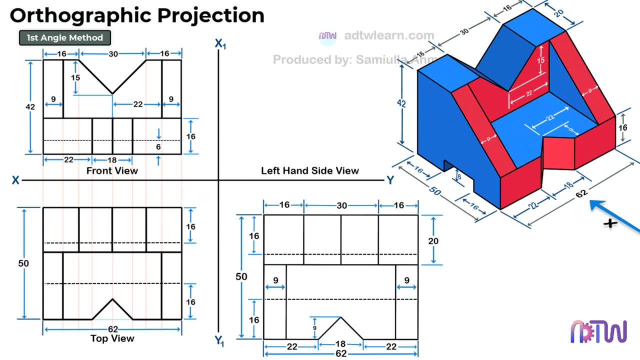 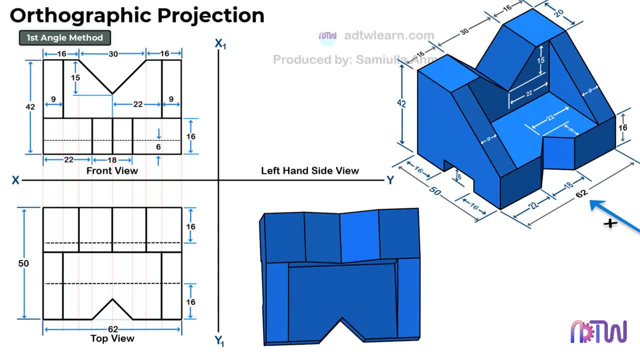 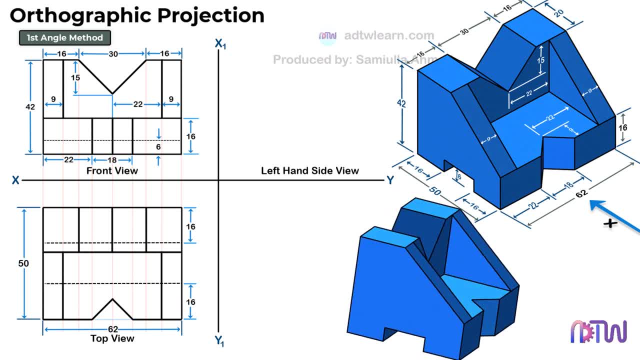 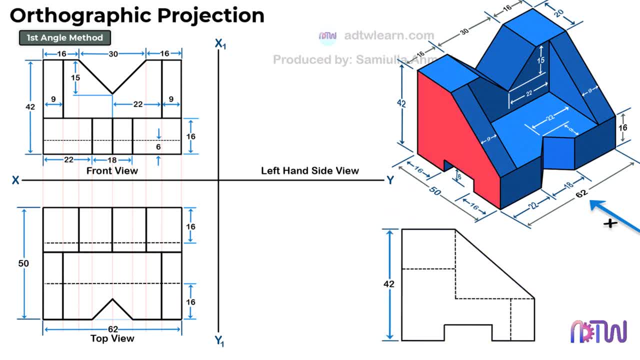 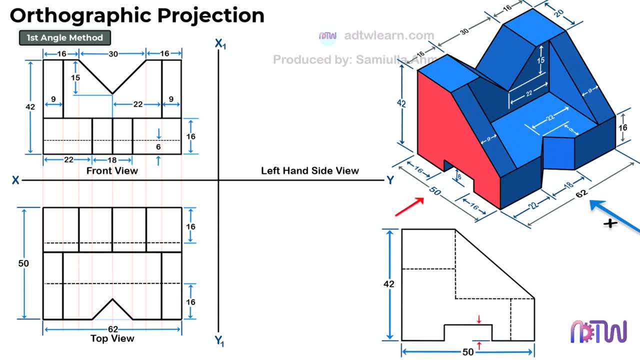 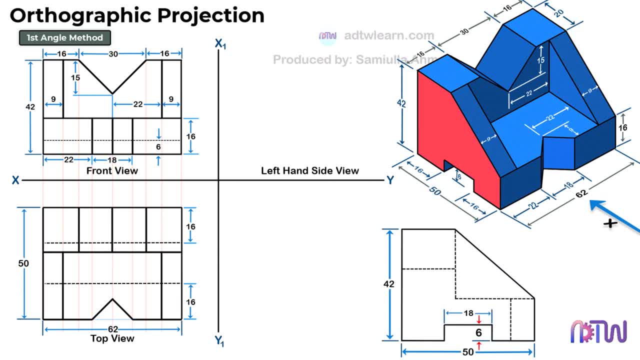 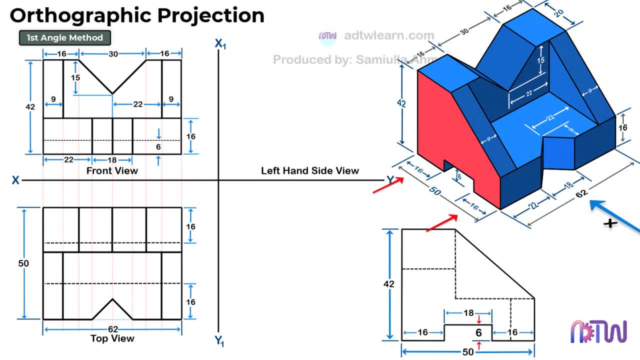 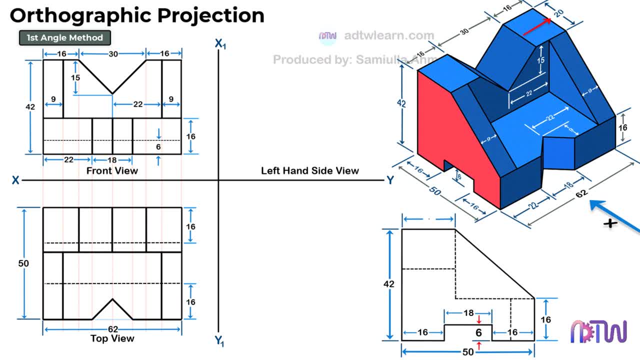 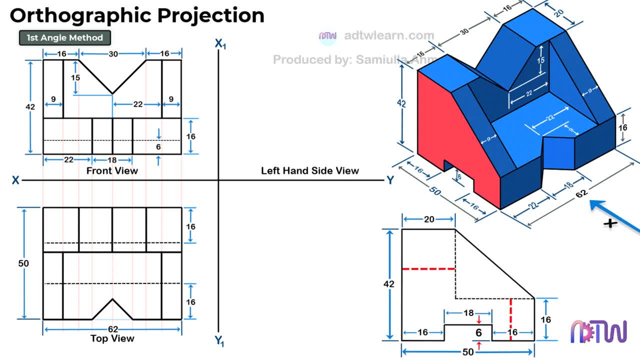 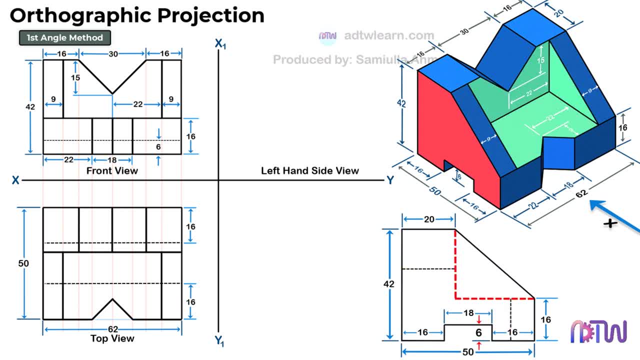 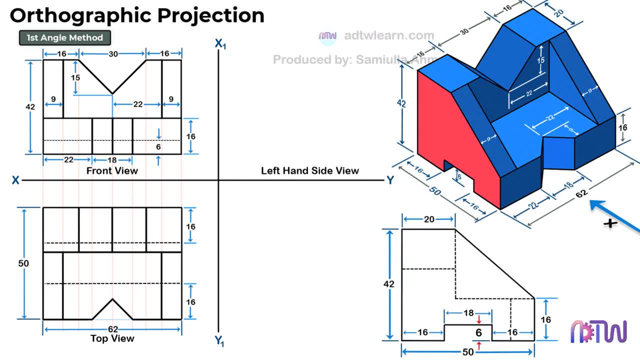 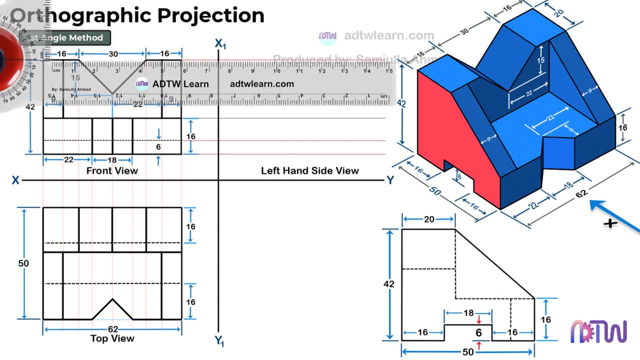 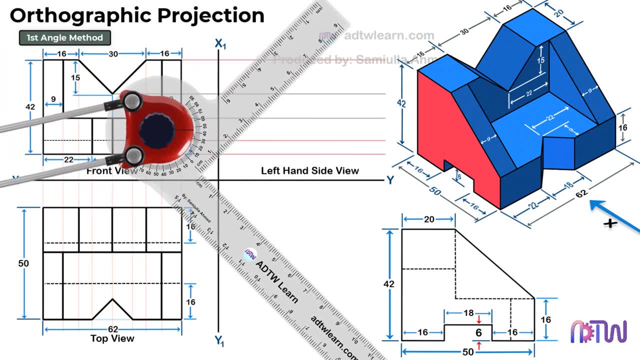 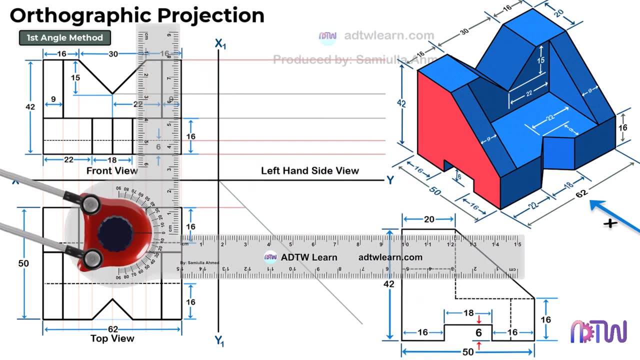 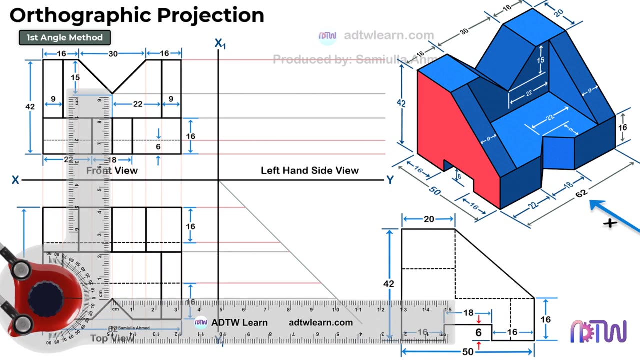 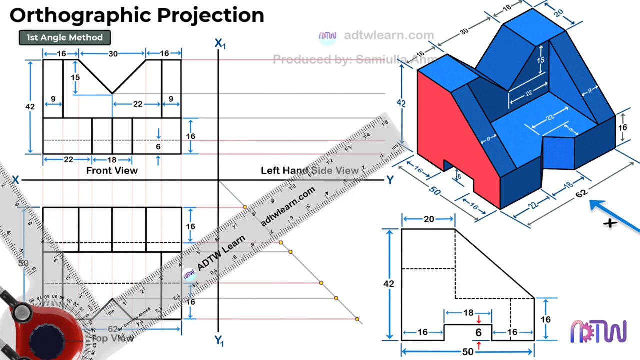 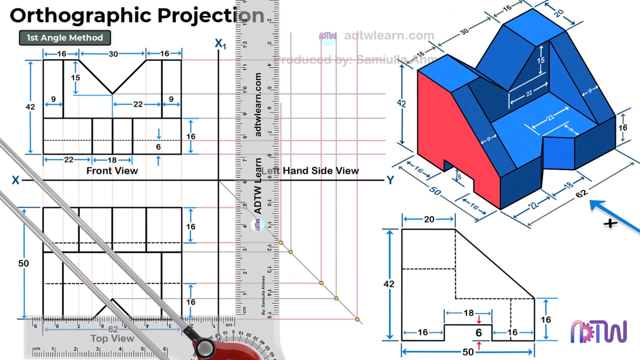 After this, draw the reference lines from the top view. To get the reference lines from the top view, we will draw an inclined line at 45 degrees. Next, draw the horizontal lines from the corner points of the top view. After this, draw the vertical lines from each of these points. 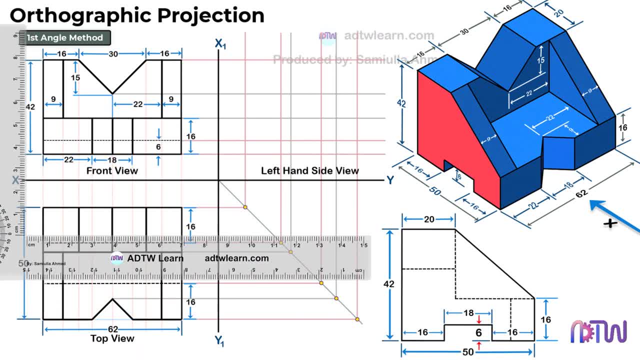 These reference lines will help us in drawing the left-hand side view. To construct the left-hand side view: To construct the left-hand side view: To construct the left-hand side view, Draw a vertical line of 42 mm, whose length will equal to the distance between these two lines. 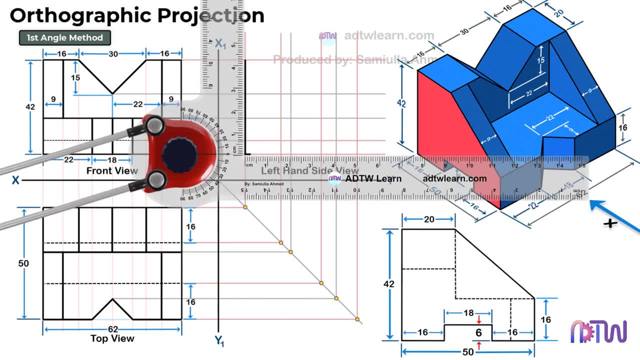 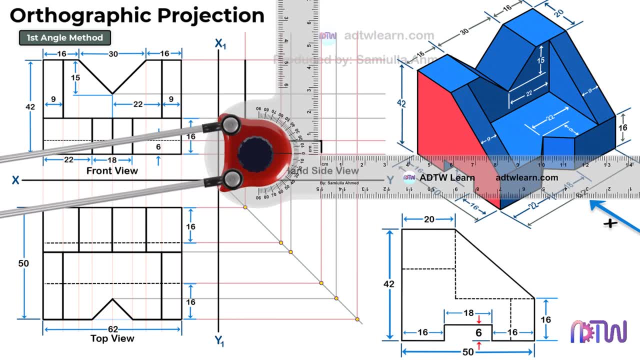 After this, draw a horizontal line of 16 mm, Then a vertical line of 6 mm, A horizontal line of 18 mm, A vertical line of 6 mm And at last, a horizontal line of 16 mm. Next, draw a 16 mm vertical line from this end point. 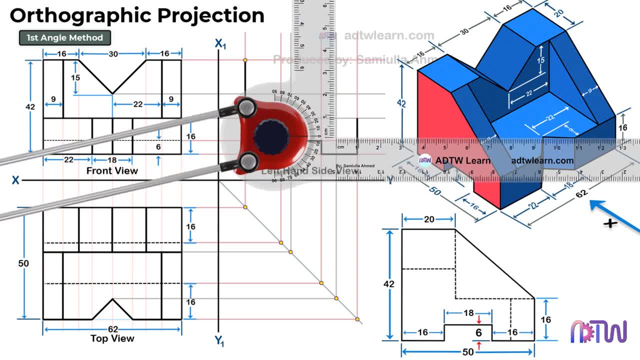 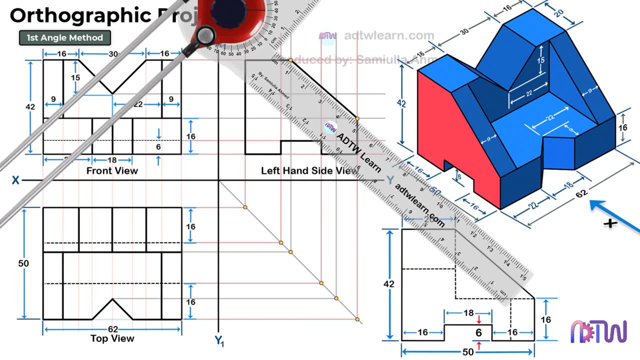 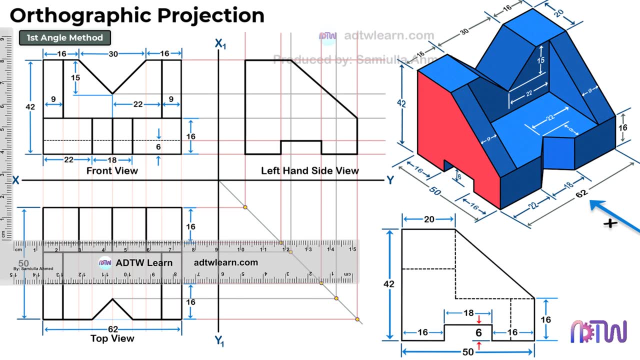 Draw a 20 mm horizontal line from this end point And join these two end points. Therefore, we got the outline for the side view. After this, we need to draw the dotted lines representing the hidden features of the object. Draw a dotted line on this horizontal line as shown.